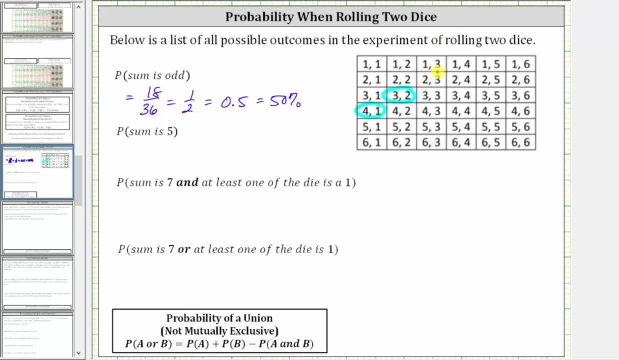 Four and one have a sum of five. three and two have a sum of five. two and three have a sum of five, and so do one and four. So there are four favorable outcomes out of a total of 36 possible outcomes. The probability the sum is five is 4- 36,. 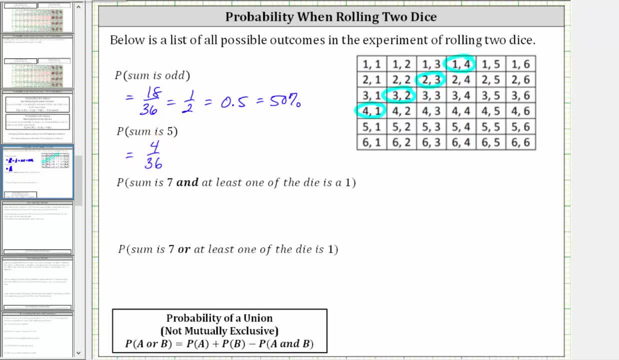 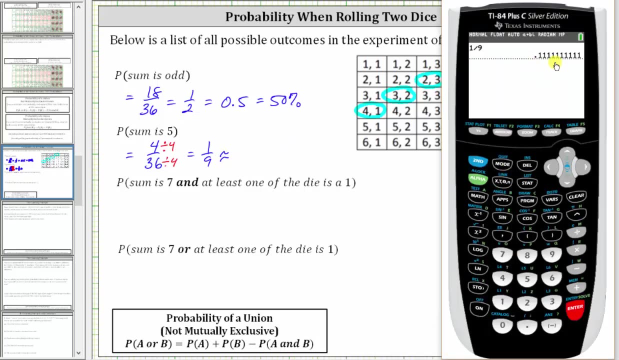 which does simplify. The greatest common factor between four and 36 is four. To simplify, we divide both by four, which is equal to 1. 9th, and let's find the decimal and percentage as well. One divided by nine is 0.1,. 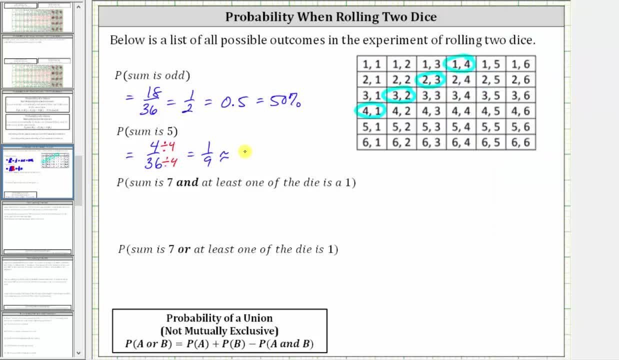 repeating to four decimal places, This would round to 0.1111, which is equal to 11.11%. Next, we're asked to find the probability. the sum is seven and at least one of the die is a one, So both of these must be true. 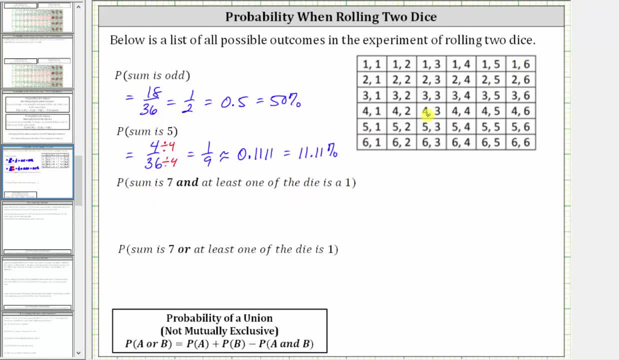 in order to be a favorable outcome. Notice along this diagonal: here the sum is seven, but only the six and one and one and six have a sum of seven and one of the die shows a one, and therefore there are only two favorable outcomes out of a total of 36 possible outcomes. 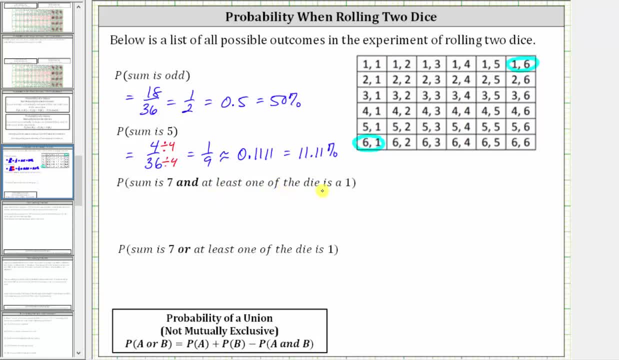 The probability, the sum is seven and at least one of the die is a, one is 2, 36th. Again, we don't count five and two, four and three, three and four and two and five as favorable outcomes because, while the sum is seven, 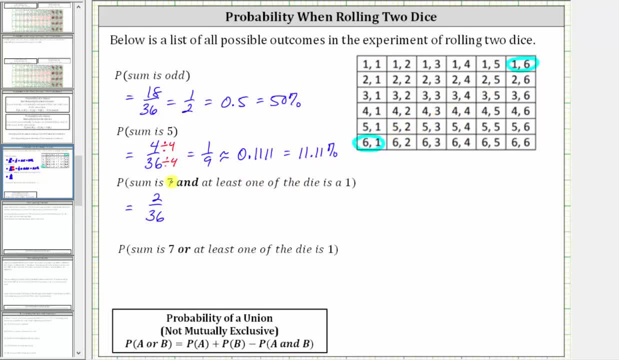 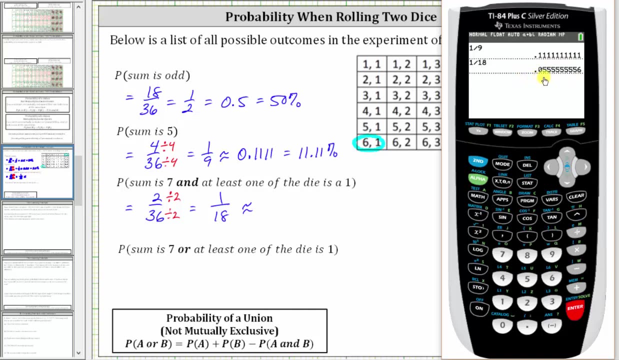 at least one of the die is not a one. So the probability is 2, 36th, which does simplify. Dividing both by two, the simplified probability is 1, 18th, which is a decimal to four decimal places, is approximately 0.0556.. 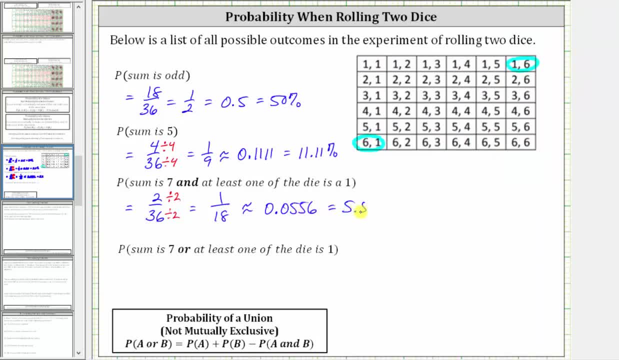 Which is equal to 5.56 percent. And for the last example, we're asked to find the probability. the sum is seven, or at least one of the die is one. So because of the or, if either is true, we have a favorable outcome. 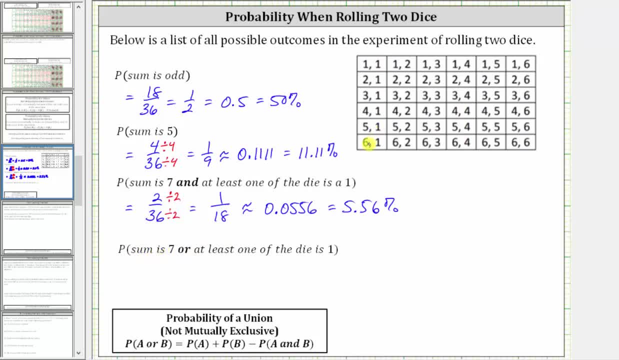 Let's first circle the outcomes where the sum is seven, which would be this diagonal here: Six and one, five and two, four and three, three and four, two and five and one and six. all have a sum of seven. And now I'll circle the remaining favorable outcomes.